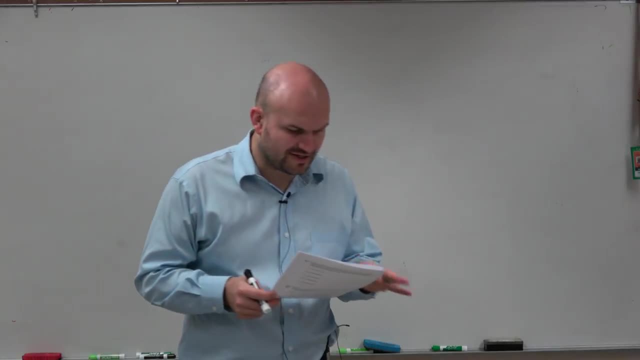 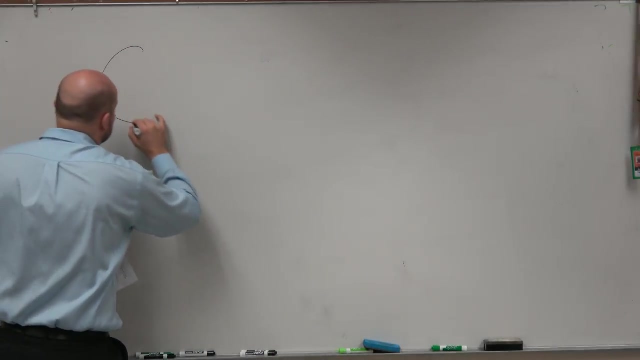 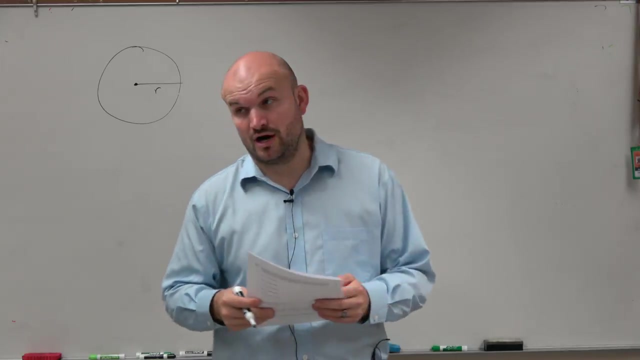 Alright. so this problem states that the radius of a circle is increasing at a non-zero rate. So immediately I am going to draw a circle, I'm going to represent a radius, and I know that this is expanding, and so therefore I automatically know that I'm going to have 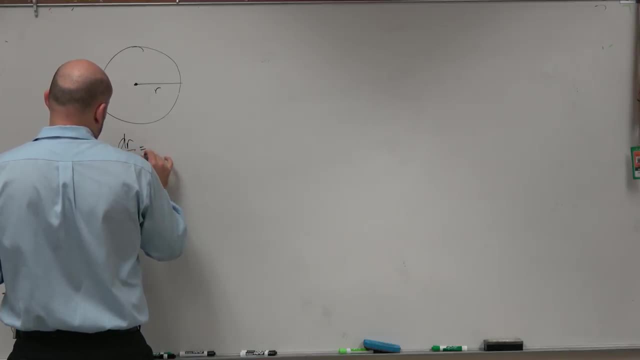 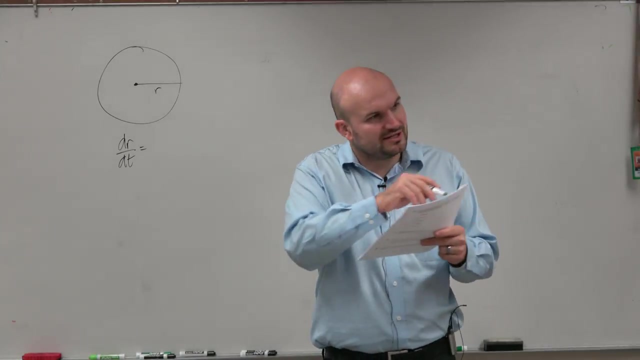 dr dt. Right, I know that I'm going to have. I want to be able to figure out this expanding like that's just the first sentence I wrote. you know, technically I'd probably just like underline it, but I know this is going to be somewhere a part of this problem, right? 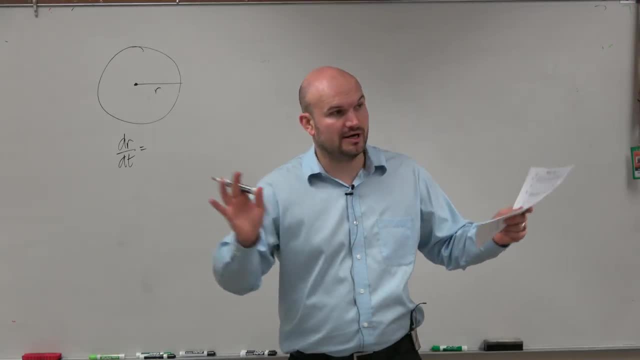 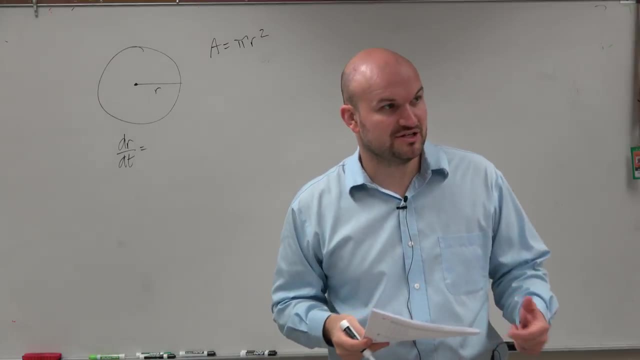 It says the rate of increase in the area of the circle. so, oh, area of the circle. alright, let's write that out there. area equals pi r squared right Real quick. just mentions area. I don't know if I'm going to need to use this, but I might, so I'm just going to. 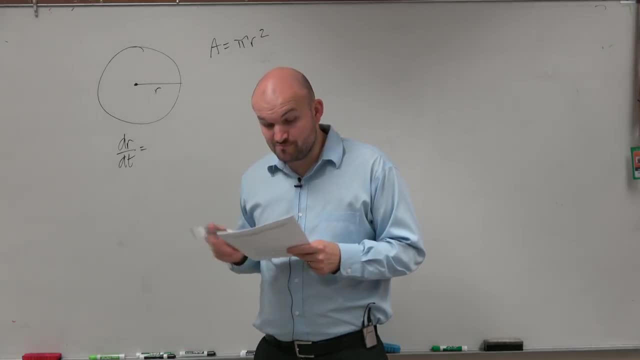 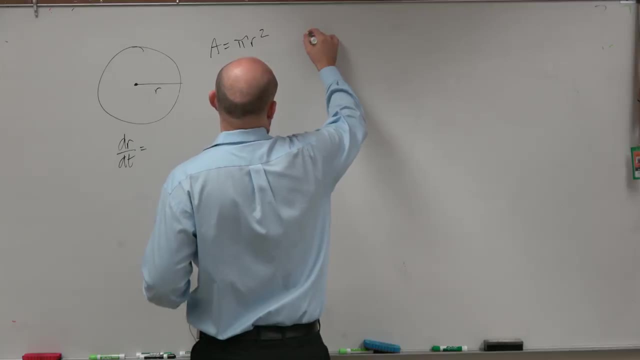 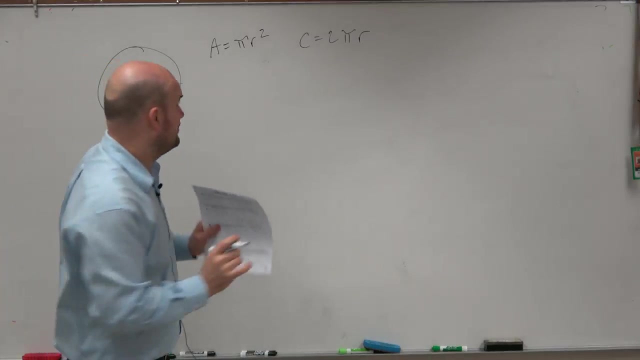 write it down: Rate of increase in the circle is numerically equal to of the increase of the circumference. oh okay, circumference. circumference equals 2 pi r. Now again, what did they say? they were equal, They were numerically equal. that means a is equal to. 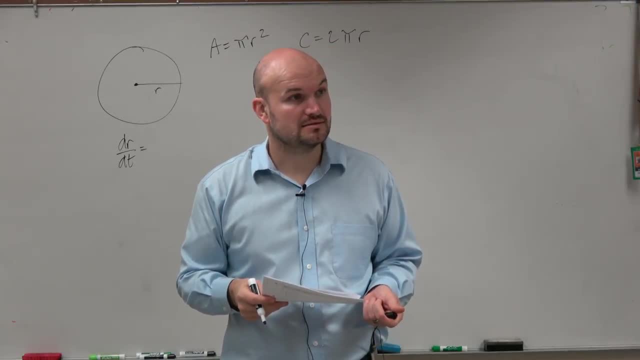 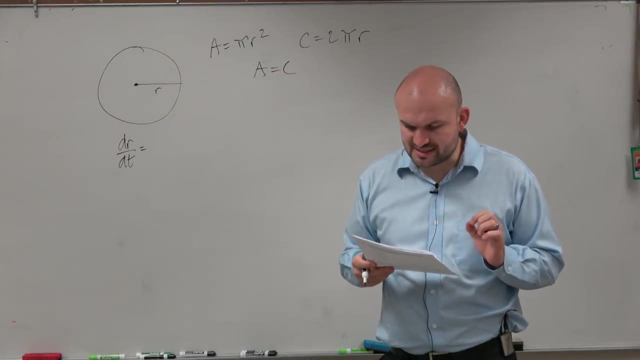 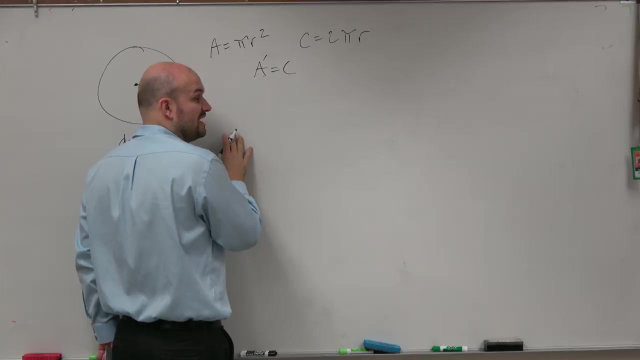 c correct. Alright so, but it says the rate of increase in the area of the circle is numerically so. that's important. actually, it's not a equals c. the rate of increase of the area is c Is equal to the rate of the increase of the circumference, so it's the derivative of each. 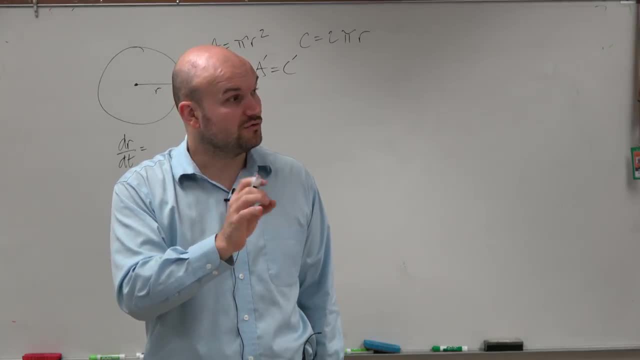 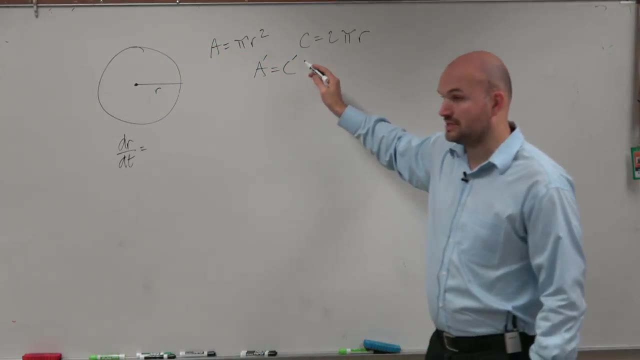 of those right Didn't say the area is equal to the circumference. it says the rate of change in the area is equal to the rate of change in the circumference. So if I'm trying to find a prime is equal to c prime. well, first thing we want to do is let's figure. 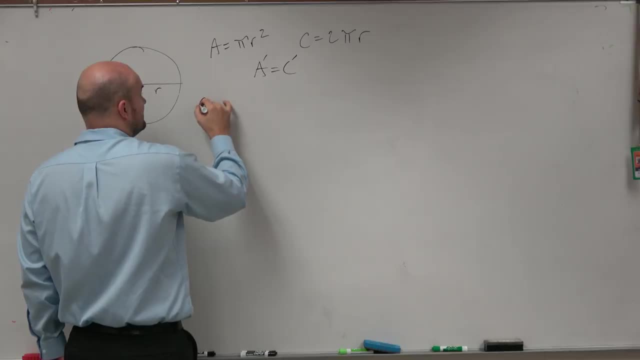 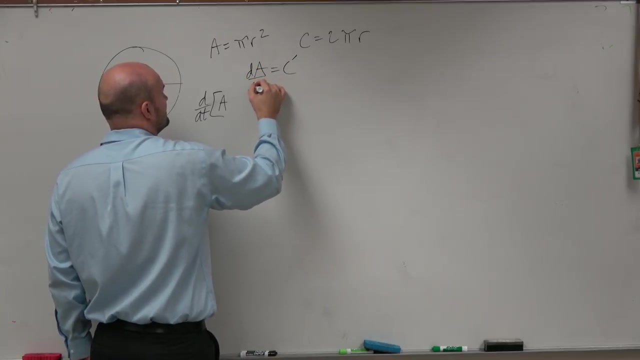 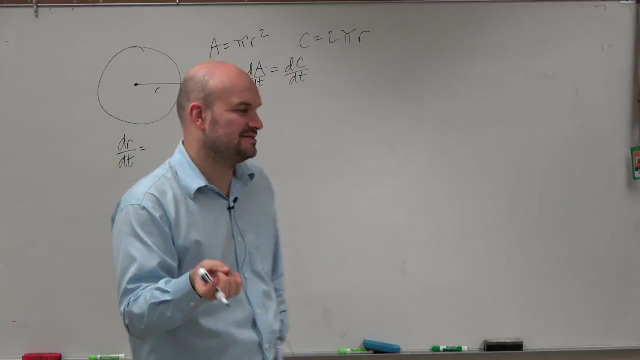 out what a prime is now with respect to t, and actually I should probably write this as d a d t. it's actually a recurrence- d c, d t. right, It's not really a prime. it's with respect to t, so we probably should. 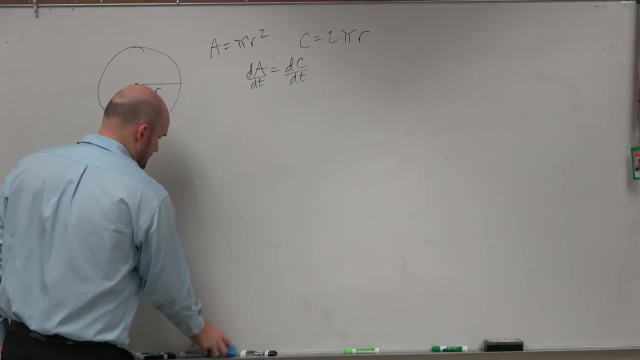 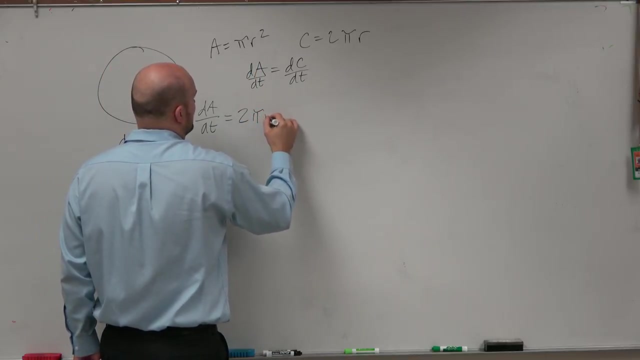 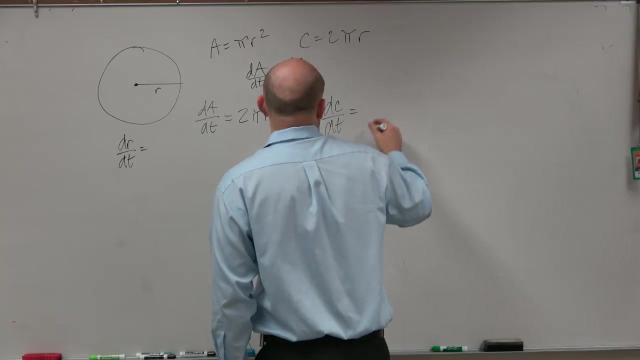 be a little bit more better mathematical with that. So therefore, let's figure out what d a d t is. In this example, that's just going to be 2 pi r d r d t, and d c d t equals 2 pi d r d t, right?